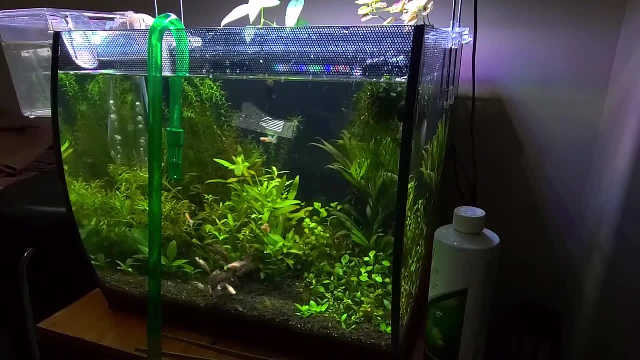 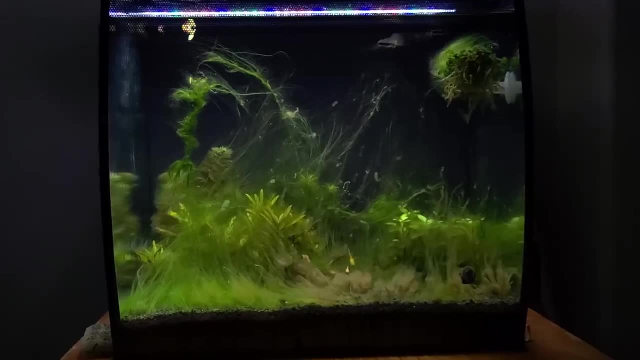 Which brings us to the weaknesses of EI dosing. You MUST reset nutrient levels through massive water changes of 50% or more every week. Failure to do so can significantly increase the risk of algae growth due to nutrient imbalances. I did mention that there are two main methods. 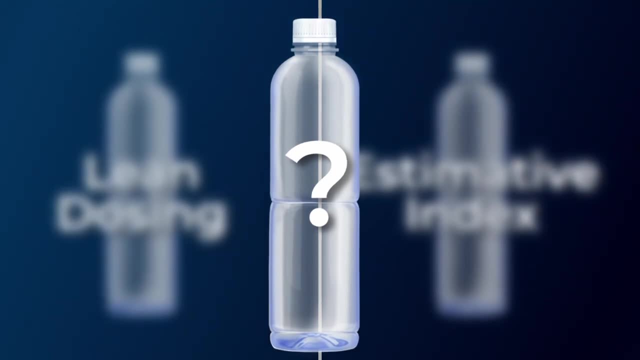 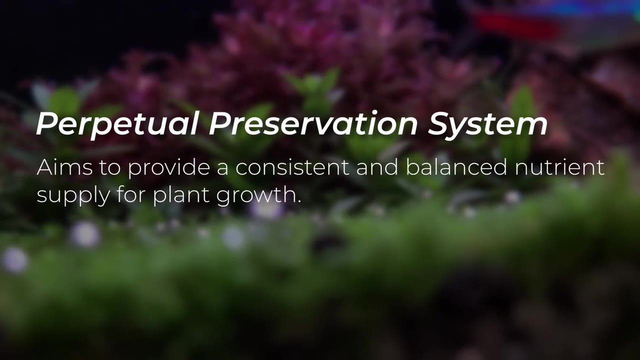 of fertilization. However, there is a third, lesser-known system known as the Perpetual Preservation System or PPSM. This system is known as the Perpetual Preservation System, or PPSM- PPS for short. PPS aims to provide a consistent and balanced nutrient supply for plant growth. 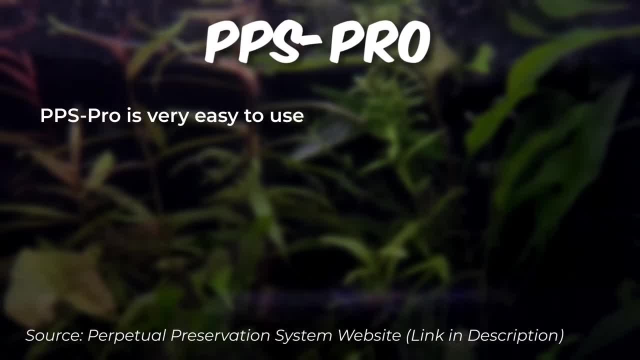 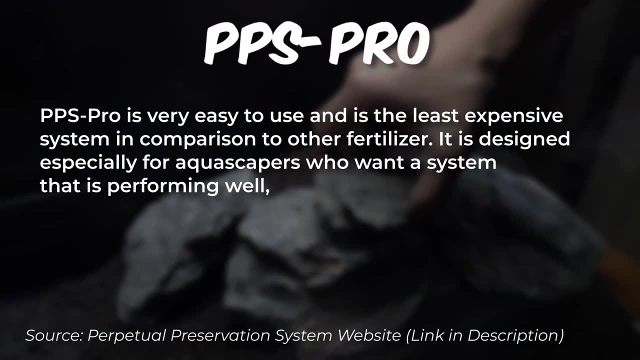 It comes with two different categories. PPS Pro is very easy to use and is the least expensive system in comparison to other fertilizers. It is designed especially for aquascapers, who want a system that is performing well, doesn't need testing and tweaking, works with all lights and. 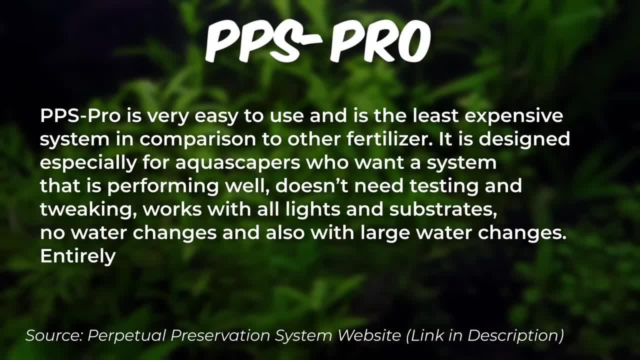 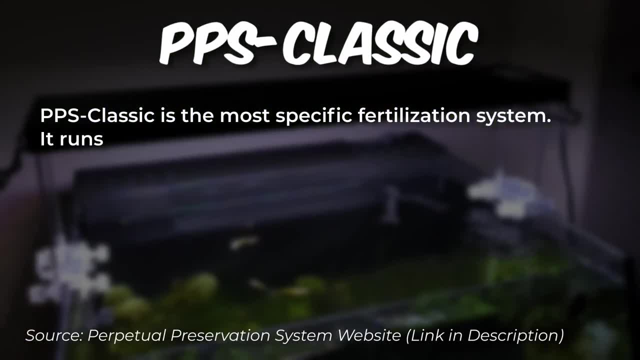 substrates, no water changes and also with large water changes, Entirely 100% planted aquariums with reasonable fish load. PPS Classic is the most specific fertilization system. It runs aquariums for years and also with water changes at regular intervals As a routine. it does involve some 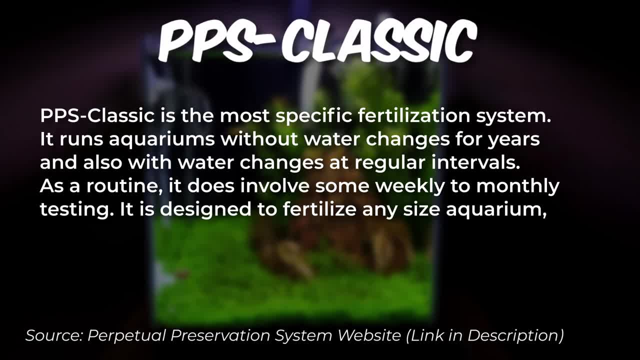 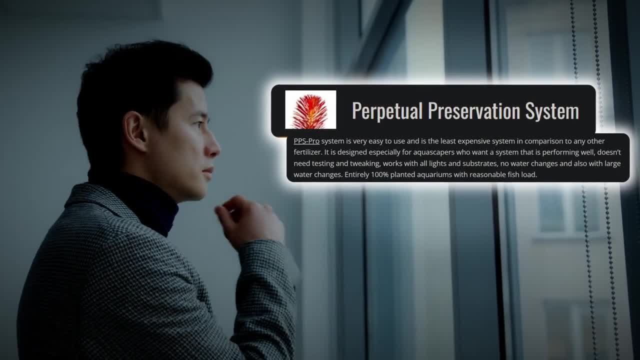 weekly to monthly testing. It is designed to fertilize any size aquarium with any light intensity and any substrate. FYI, I have never tried this type of fertilization method before, but the description really makes me want to. The good thing about this system is that you. 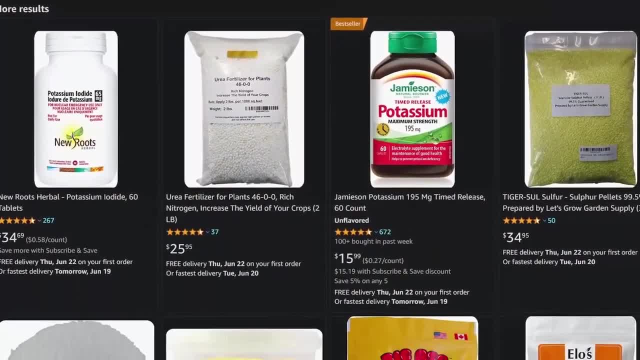 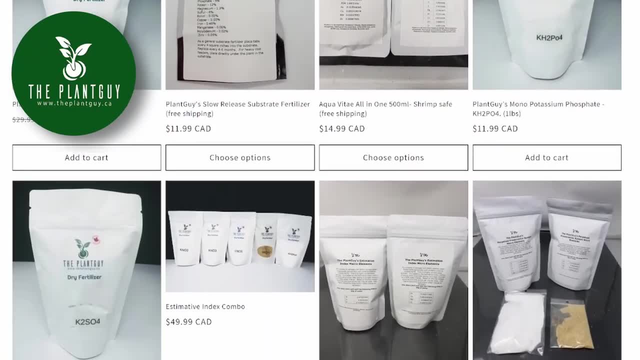 can completely DIY it. The only challenge is that you have to source the macro and micronutrients for yourself or find a supplier who sells the components for the system. As far as I know, the plant guy is a seller for us Canadians, Not sponsored, by the way. 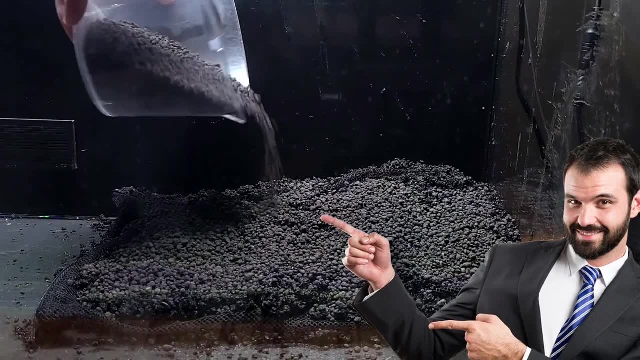 Considering these three systems. the PPSM and PPSM are very similar in terms of their systems. Which one should you go with? Just because you have a nutrient-rich substrate does not automatically mean you should choose Lindozan. There is more to consider. First off, 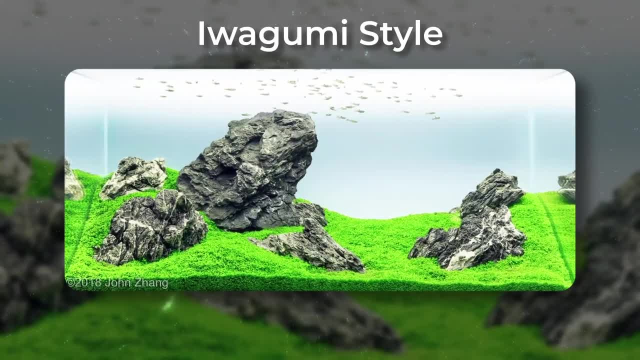 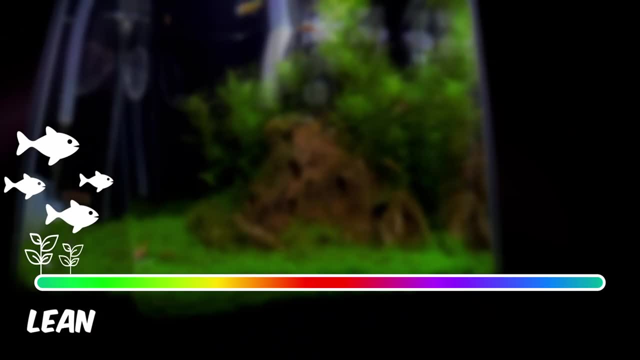 you will need to reflect on your livestock buyer load and the type of aquascape you have. If you have an aquarium with a large buyer load and low density of plants, you may want to choose a more leaner method, as your buyer load will contribute to the amount of nutrients in the water column. 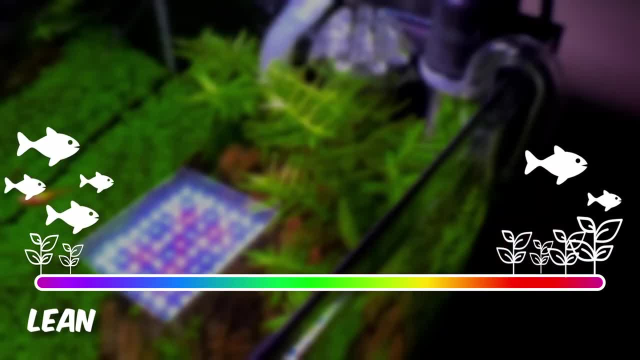 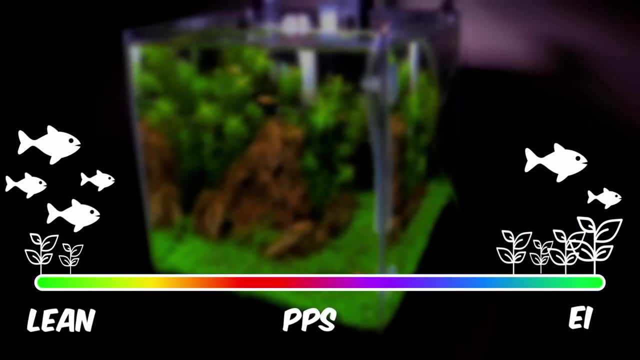 If you have a tank with a small buyer load and a large density of plants, you may want to lean towards EI method. instead, You can try PPS method, as it would fall right in the middle. Again, this is just my experience with PPS, so let me know how it goes for you if you choose it. 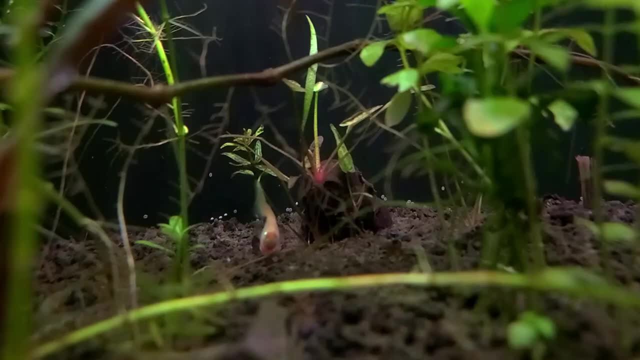 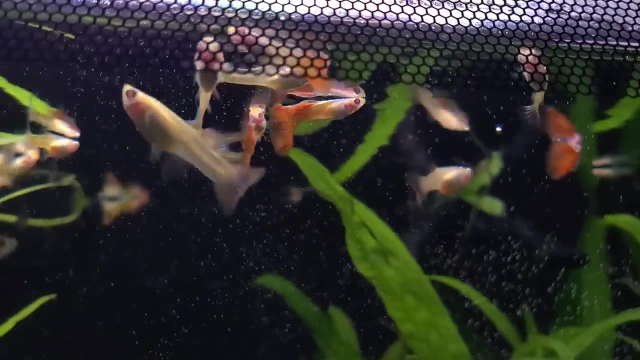 This concept is what I believe to be one of the main reasons why my dirted fluvoflex inevitably failed. My theory was: more plants equals more nutrients needed, which is why I went with EI. I did not take my large guppy buyer load into consideration In terms of aquascapes.